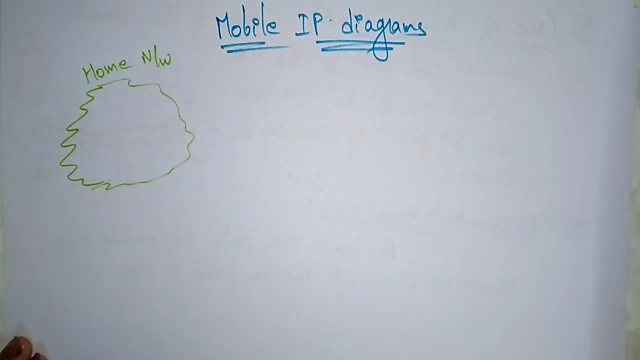 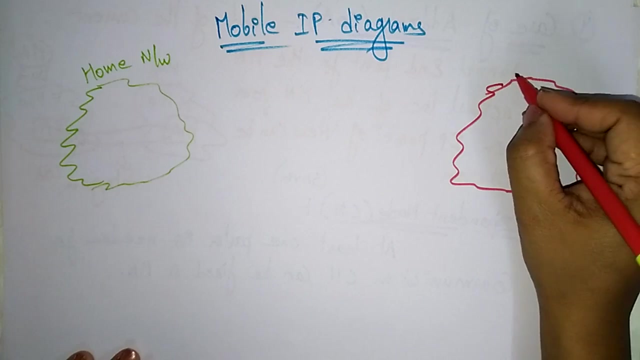 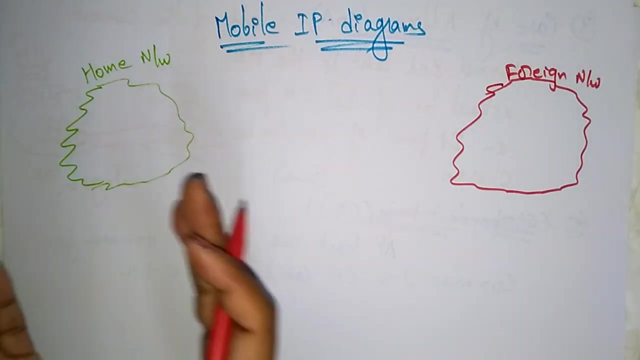 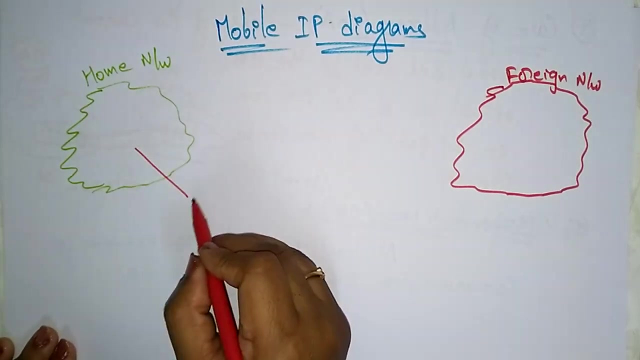 Home network And somewhere else you are having the foreign network. So this is a. let's take this is a foreign network, So means starting at position, your mobile load is at your home, So in your home you are having one router. Okay, so one router will be there. Let us take one router. 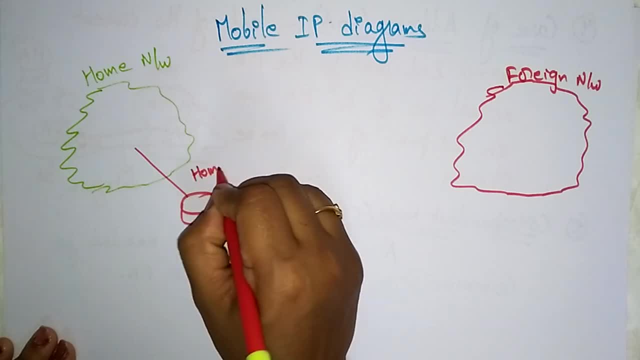 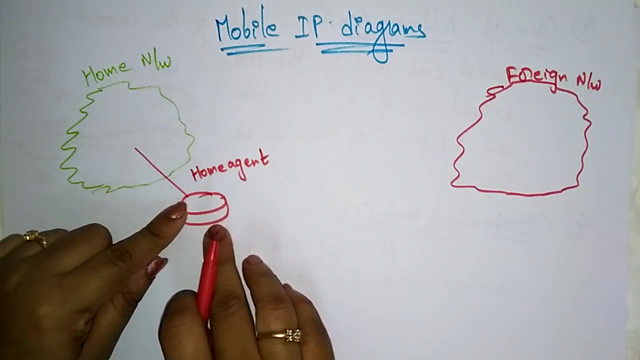 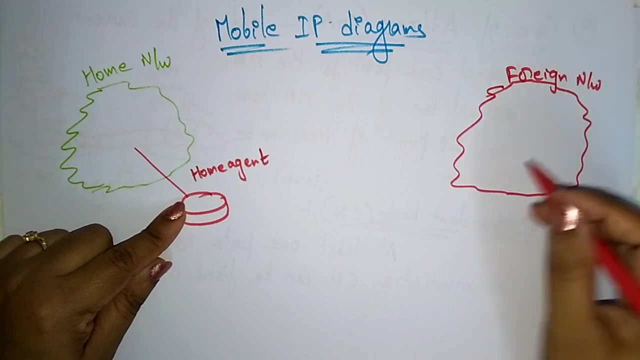 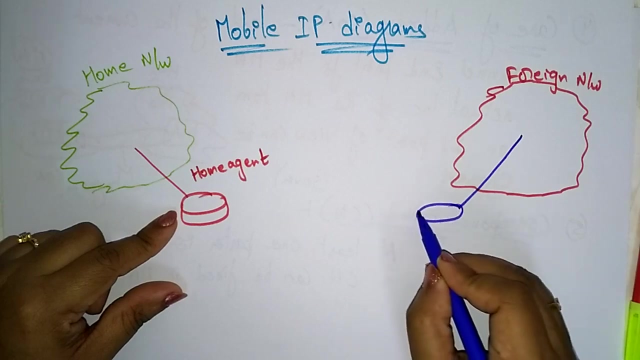 So this router you call it, Call it as a home agent. Your home network will be connected to one router. that is a home agent. This home agent will register your mobile node. Okay, so for foreign network is also having one router, That is, the foreign agent is also having one router. So this is a foreign route for an agent. 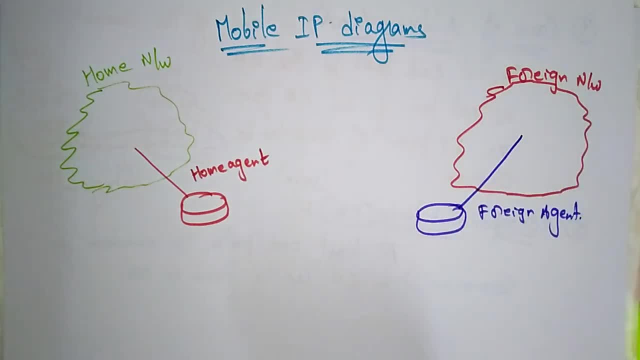 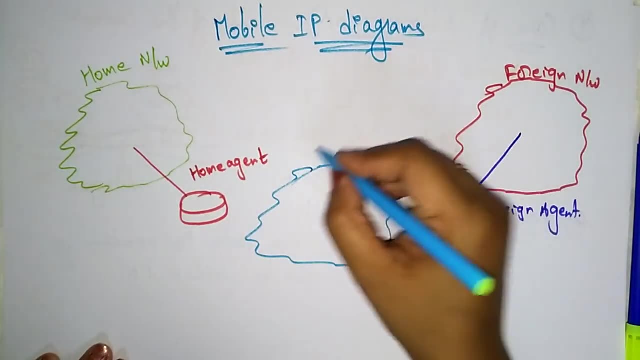 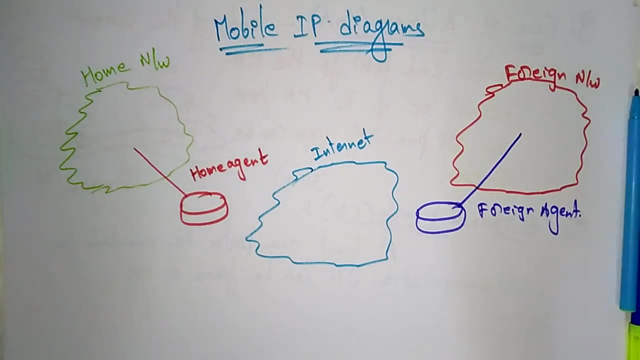 Which maintains the current locations of this mobile node. So in between we are having an internet, So this is an internet, Excuse me. So in the internet you are having a tunnel, So this tunnel is used to pass your data gram. 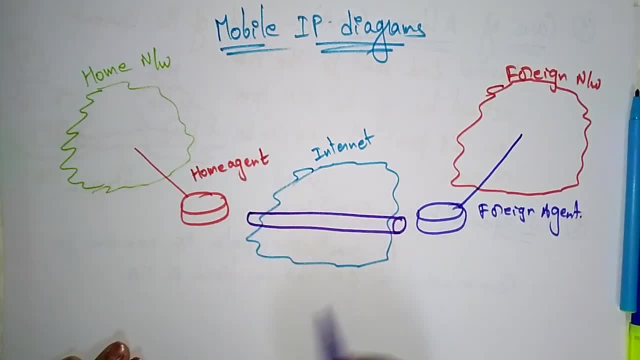 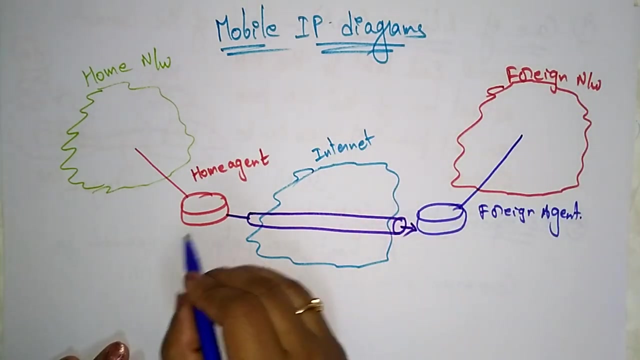 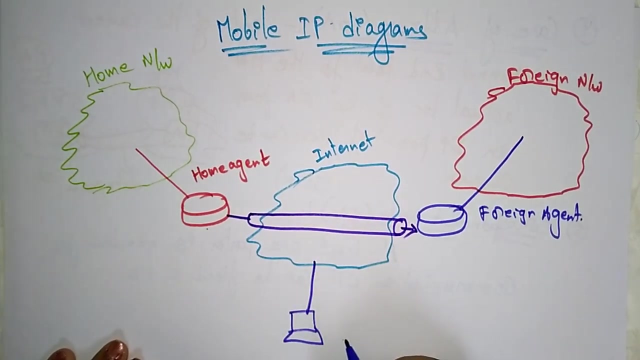 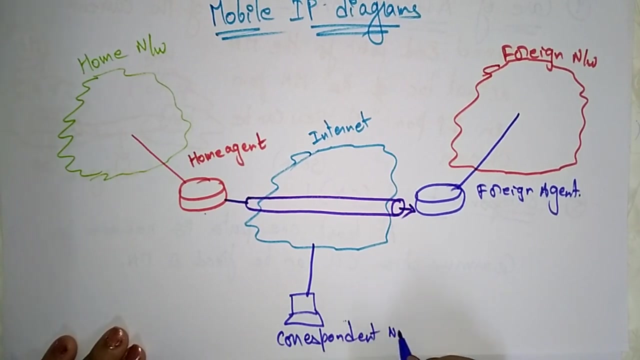 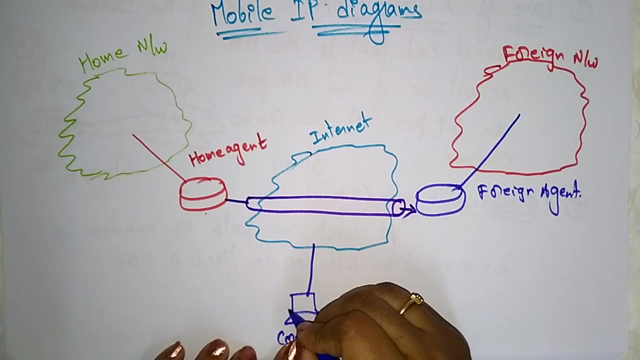 Okay, this is going to pass your data gram, So in between that, one correspondent node will be present. This is a correspondent node. Let us take a server or anything else, So this is a correspondent node, Correspondent node. Excuse me, Okay, so now let us see what exactly it is doing. First, what it is doing: The first the correspondent node is sending information to the home agent. 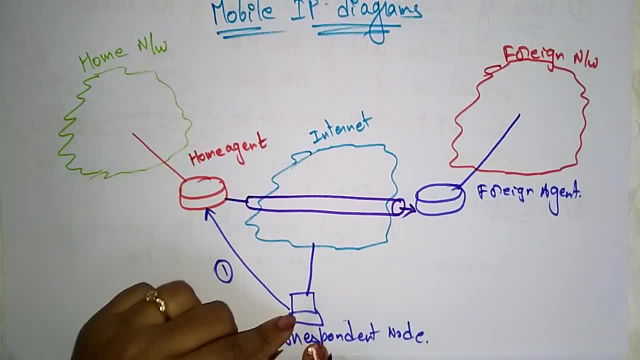 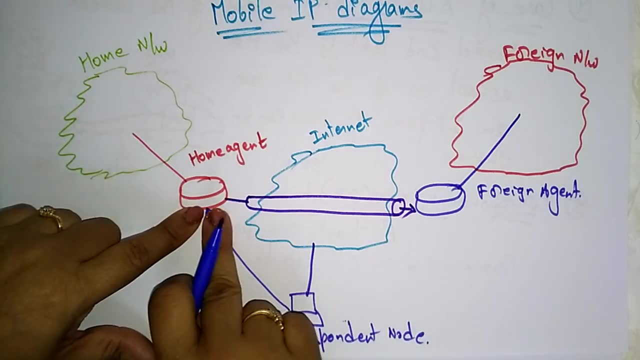 This is the first step, means it is with the help of this correspondent node. You are first registering your mobile node at the home location home network. So now my mobile node is moving from my home network to the foreign network. So now my mobile node is moving from my home network to the foreign network. 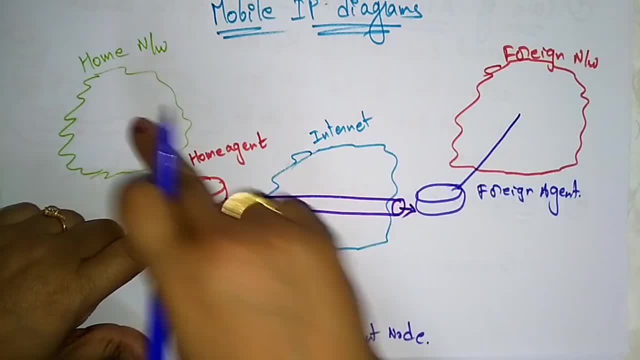 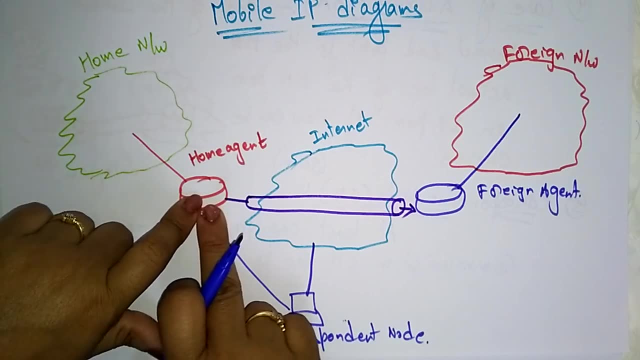 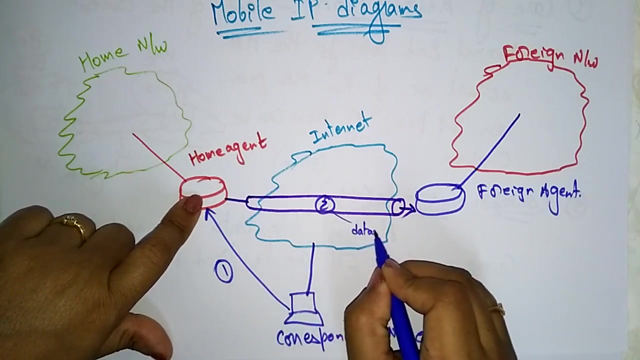 my home network to the foreign network. okay, somewhere from hydropower to bangalore i am moving. so what it is doing, so this home agent is passing the information over the tunnel, which consisting of a datagram. a datagram will be present, this datagram consisting of some your 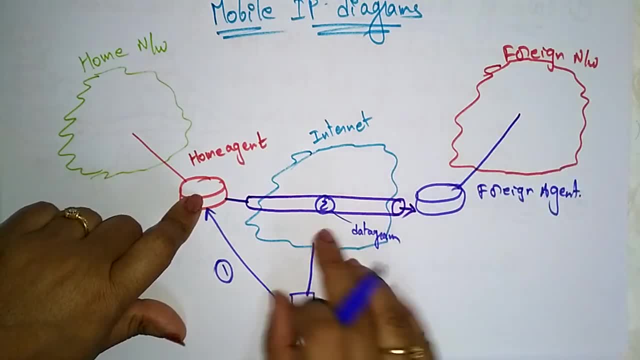 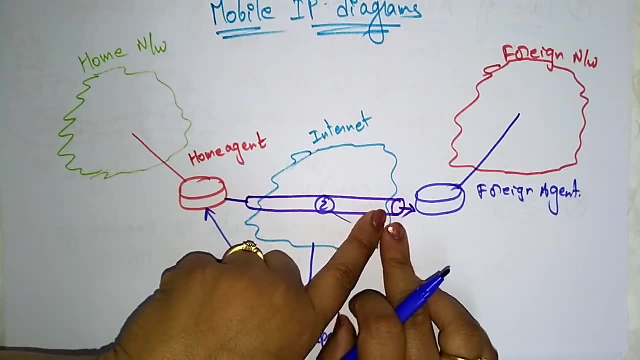 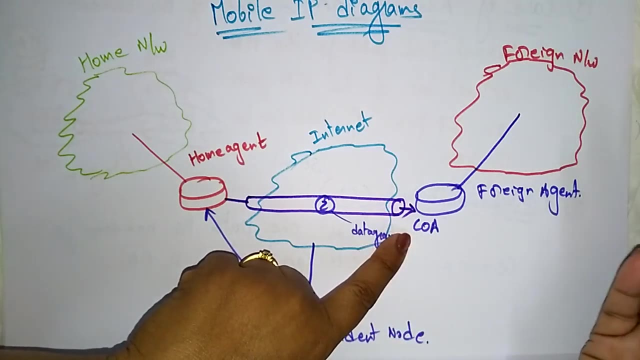 registered location and the ip address of your mobile node, and passing over the tunnel. so this is a tunnel starting point and end point. so this end point consisting of coa, the care of address, to where you have to send the letter so that care of address will be registered in this foreign 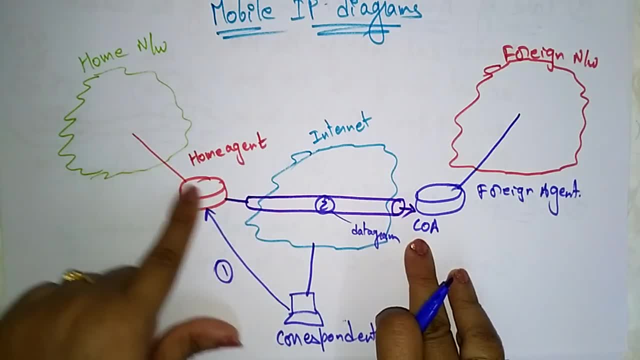 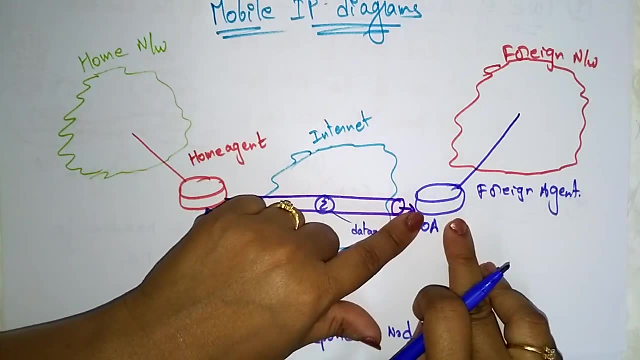 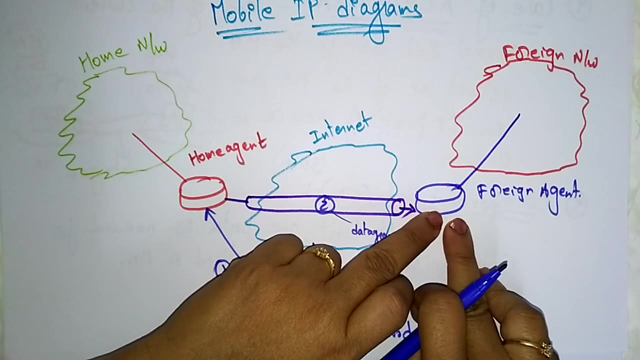 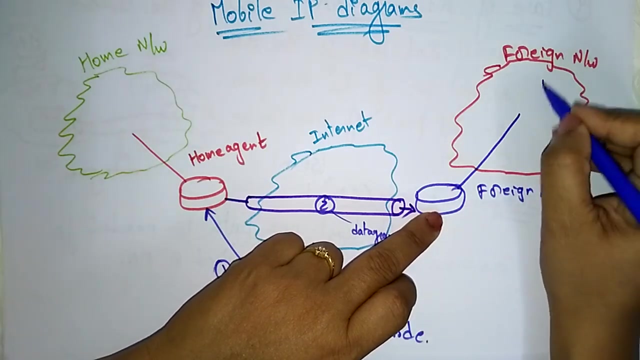 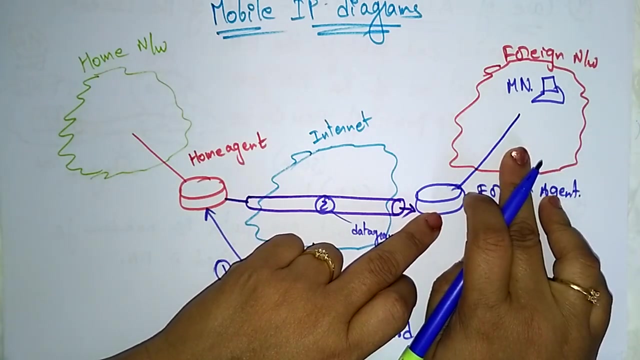 agent. so with the help of this care of address, the home agent is sending the datagram to this foreign agent. so now this foreign agent will have will receive the information regarding your mobile node, okay, and passes the informations to your mobile node that is present somewhere here. okay, the mobile node which is at the receiver site. so, first circuit it passing to. 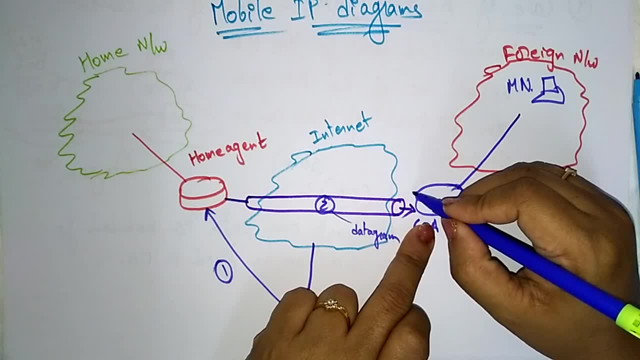 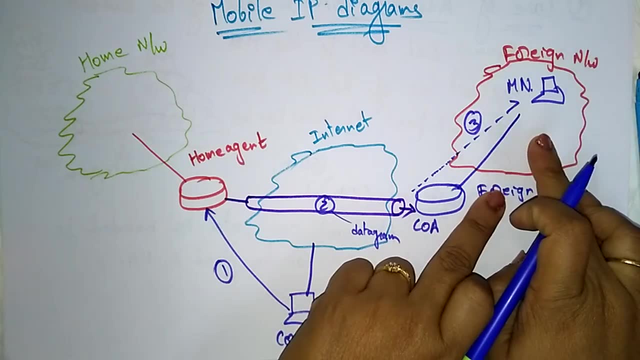 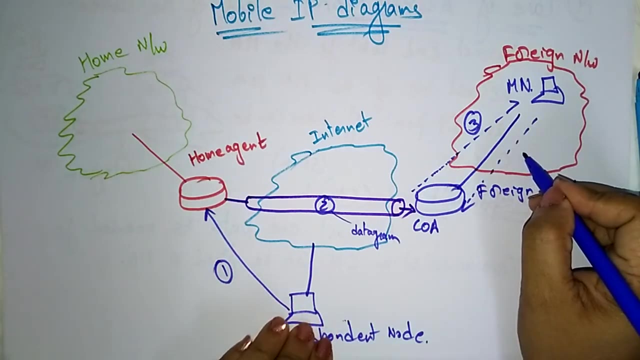 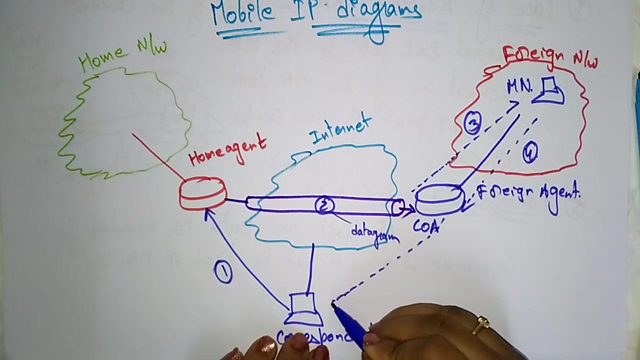 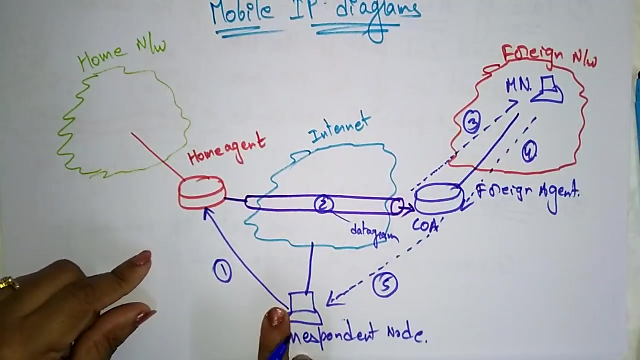 here, and next it's sending the information to the mobile node. after receiving that, the mobile node will again send back to the foreign agent, so the foreign agent sending back to the correspondent node. so again the cycle will be passing like this, just like a triangle. the information will 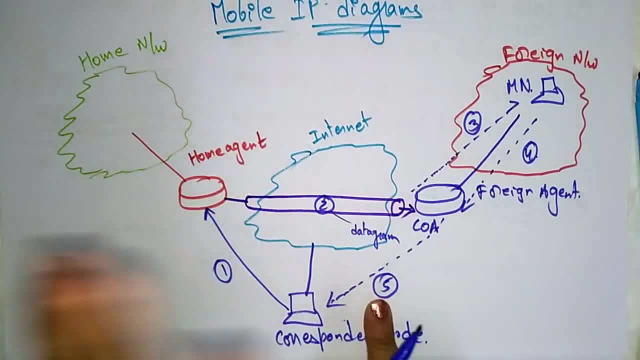 be passing like a triangle, so we also call it as a triangle IP protocol. so this is the exact a the how the mobile IP will be communicating. even though your mobile user host is moving from one place to another place, with the help of this home agent, your mobile node IP address will be constant. 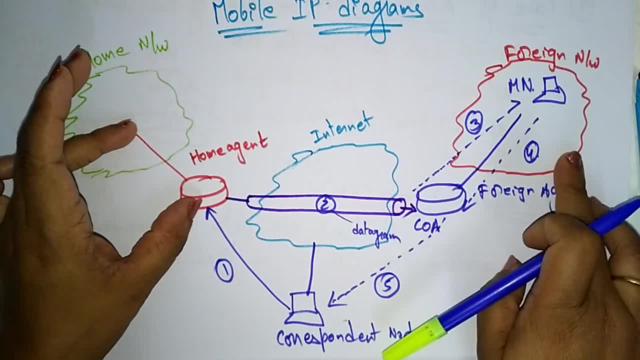 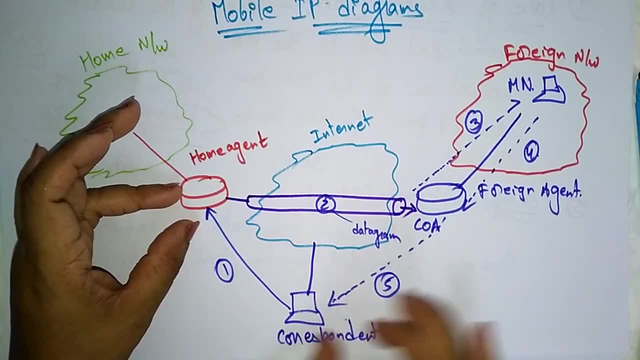 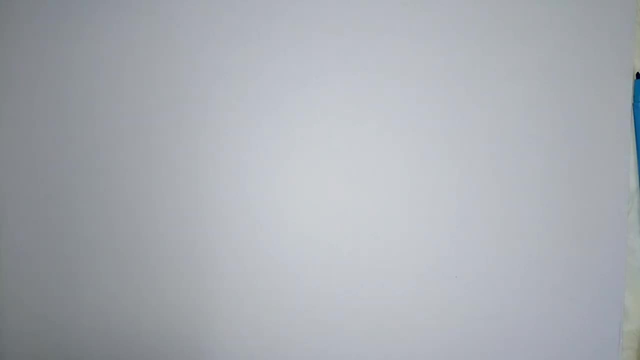 because it is communicating wherever you're going with the help of the correspondent node and the home agent. so this correspondent node is a in the layer which it can act as a server. now let me explain you the data transfer to mobile system and from the mobile system. how. 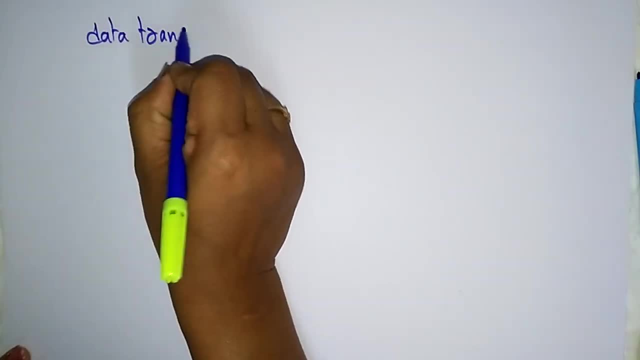 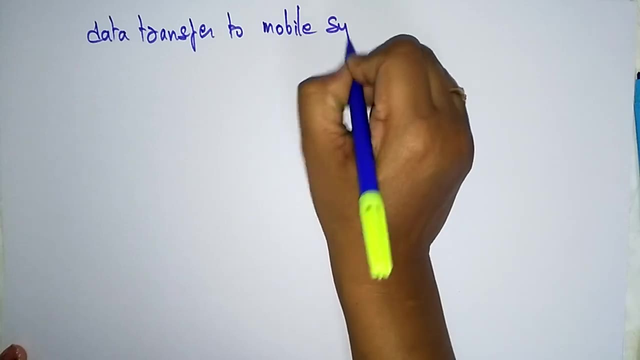 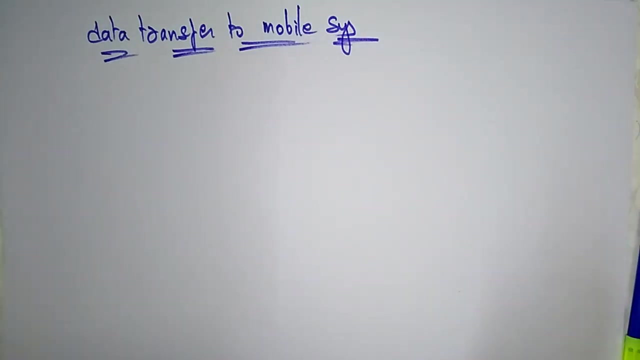 the data is transferring. data transfer to mobile system, so let us take a home network. so let us take a home network. now. let me explain you the data transfer to mobile system and from the mobile system, how the data is transferring. data transfer to mobile system, so let us take a home network. now let me explain you the data transfer to mobile system and from the mobile system. how the data is transferring. data transfer to mobile system. so let us take a home network. now let me explain you the data transfer to mobile system and from the mobile system. how the data is transferring. data transfer to mobile system. so let us take a home network. 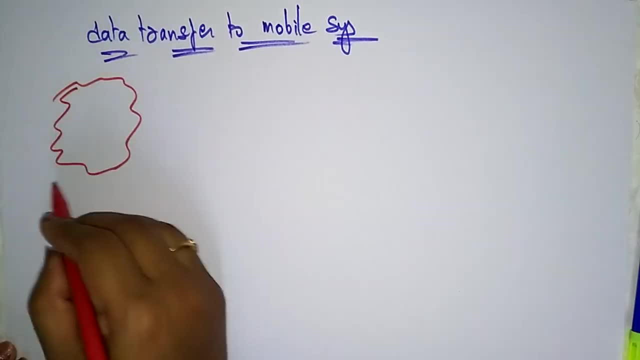 now let me explain you the data transfer to mobile system and from the mobile system. so let us take a home network now. let me explain you the data transfer to mobile system and from the mobile system. so let us take a home network now. let me explain you the data transfer to mobile system. so let us take a home network. 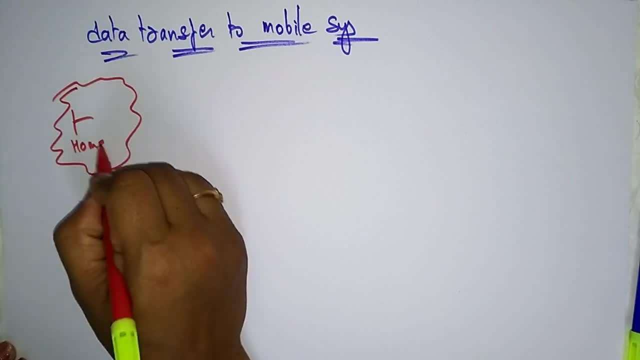 now let me explain you the data transfer to mobile system. so let us take a home network. now let me explain you the data transfer to mobile system. so let us take a home network. so here, home network is there. now let me explain you the data transfer to mobile system. so let us take a home network. 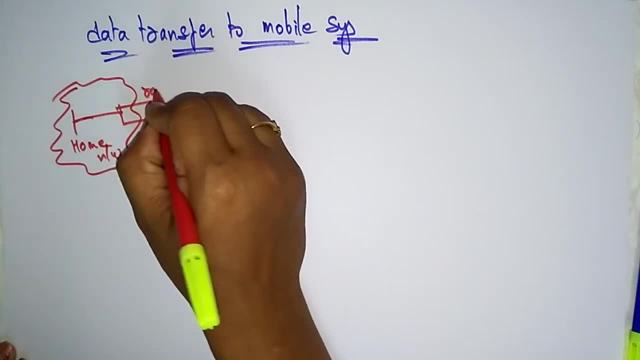 now let me explain you the data transfer to mobile system. so let us take a home network. so the home network is connected to. so the home network is connected to. so the home network is connected to. this is the router which is a home agent. this is the router which is a home agent. 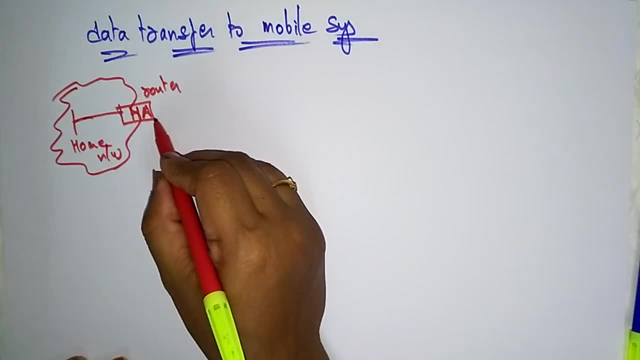 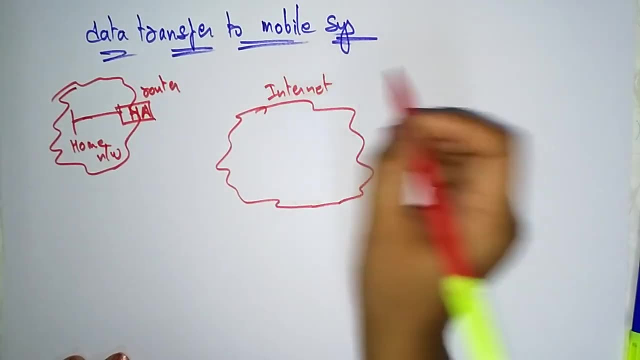 this is the router, which is a home agent. h, a home agent, h, a home agent, h, a home agent. okay, the home agent, okay, the home agent, okay, the home agent. and first let me write the pictures: this, and first let me write the pictures: this, and first let me write the pictures. this is an internet, internet, and here 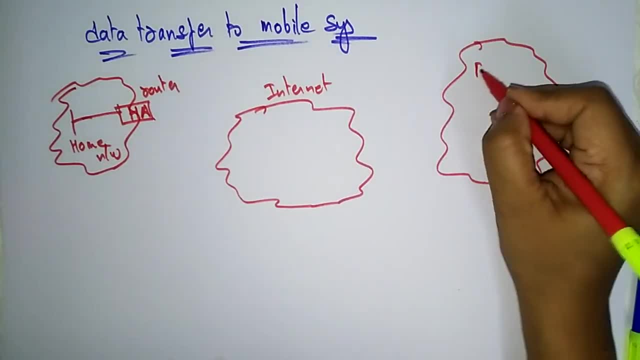 is an internet internet and here is an internet internet and here, somewhere else, a foreign network. is there somewhere else a foreign network? is there somewhere else a foreign network? is there foreign network? and somewhere here our foreign network and somewhere here our foreign network and somewhere here our mobile node is present in the ring in. 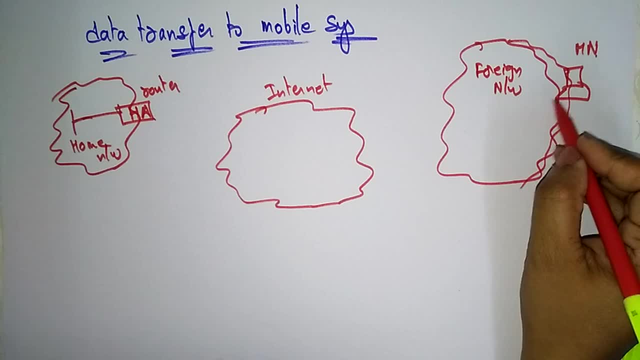 mobile node is present in the ring, in mobile node is present in the ring in this foreign network. and here the foreign, this foreign network, and here the foreign, this foreign network. and here the foreign network is connected with one router network, is connected with one router network, is connected with one router. that is a foreign agent, okay, the foreign. 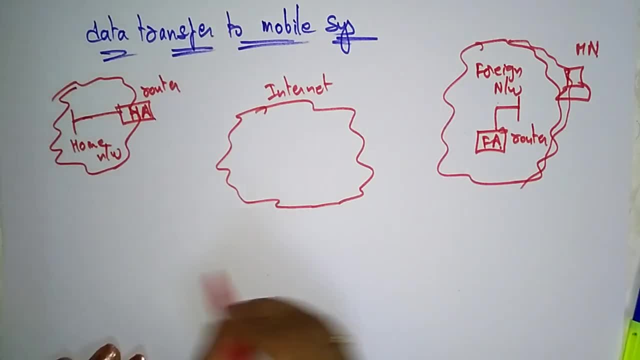 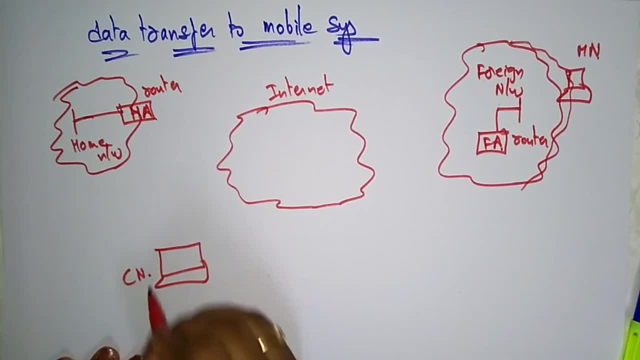 now let's say: and here one. now let's say: and here one correspondent node is present, CN correspondent node is present, CN correspondent node is present, CN correspondent node, this correspondent correspondent node, this correspondent correspondent node, this correspondent node is also having one router node is also having one router. 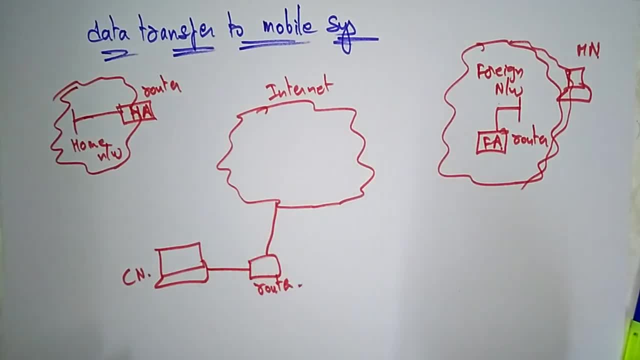 node is also having one router connected to the internet. so now let's connected to the internet. so now let's connected to the internet. so now let's see the process. so first what it is. see the process. so first what it is, see the process. so first what it is doing. first the sender sends to the IP. 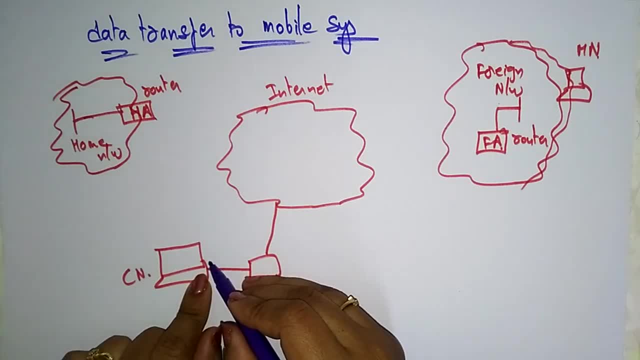 doing first the sender sends to the IP. doing first the sender sends to the IP address of the mobile node home agent. address of the mobile node home agent. address of the mobile node home agent intercepts packet. so first it sends the intercepts packet, so first it sends the. 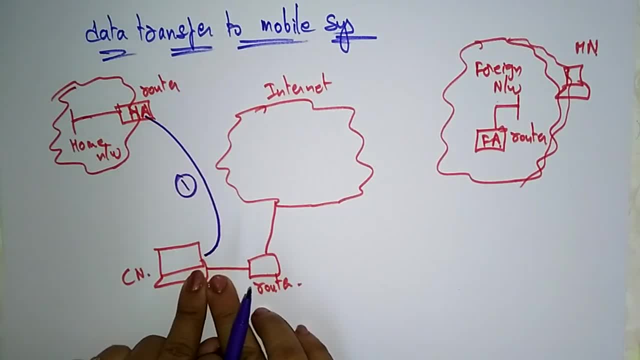 intercepts packet. so first it sends the information. the sender sends to the IP information. the sender sends to the IP information. the sender sends to the IP address of the mobile node home agent. address of the mobile node home agent. address of the mobile node home agent intercepts packet. next, the home agent. 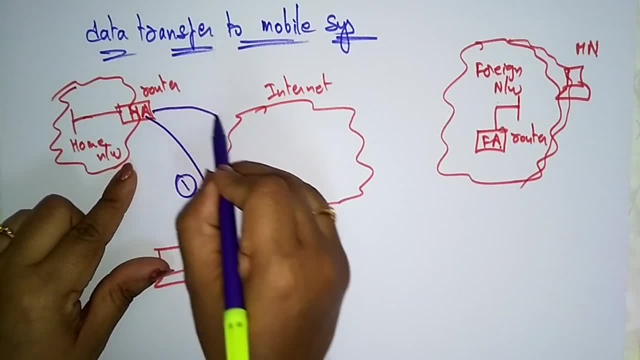 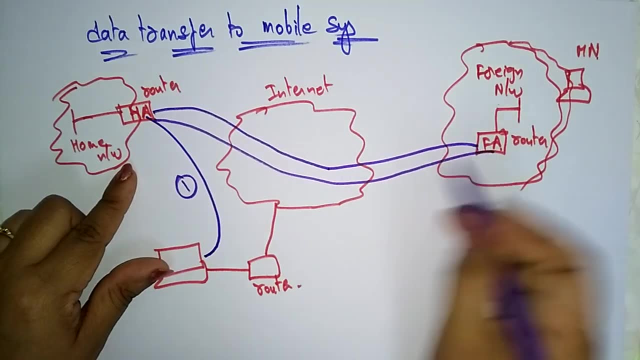 intercepts packet. next the home agent intercepts packet. next the home agent. tunnels packets to see away. so a tunnel tunnels packets to see away. so a tunnel tunnels packets to see away. so a tunnel packets to see away. so this is a tunnel. packets to see away. so this is a tunnel. 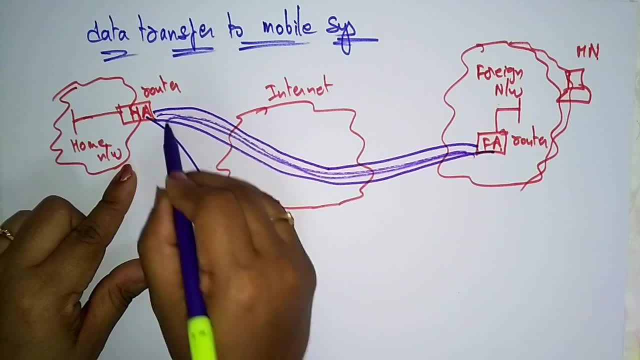 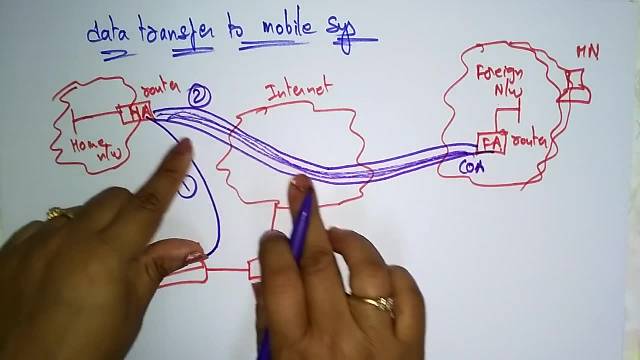 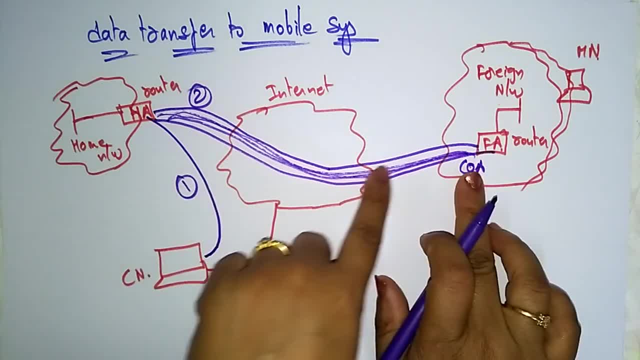 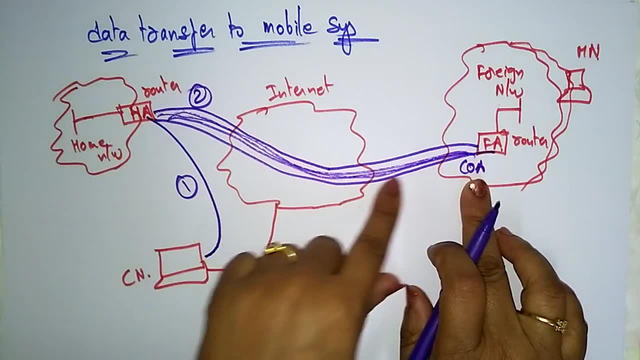 second. so packets to see away a datagram home agent tunnels packet to see what home agent tunnels packet. to see what home agent tunnels packet. to see what care of address here FA by encapsulation. care of address here, FA by encapsulation. care of address here, FA by encapsulation to foreign agent by encapsulation. so 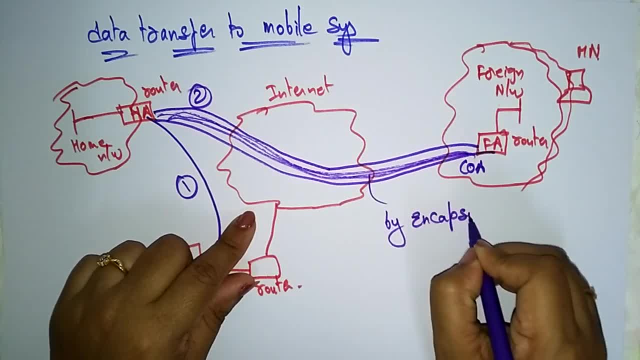 to foreign agent by encapsulation. so to foreign agent by encapsulation, so remember that. by encapsulation, so I'll remember that. by encapsulation, so I'll remember that. by encapsulation, so I'll explain about this encapsulation also in. explain about this encapsulation also in. 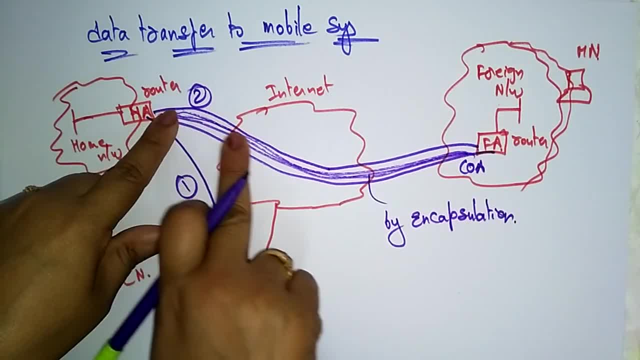 explain about this encapsulation also in the tunnel. so the COA, the datagram is the tunnel, so the COA, the datagram is the tunnel, so the COA, the datagram is passing over the tunnel to COA. by passing over the tunnel to COA, by 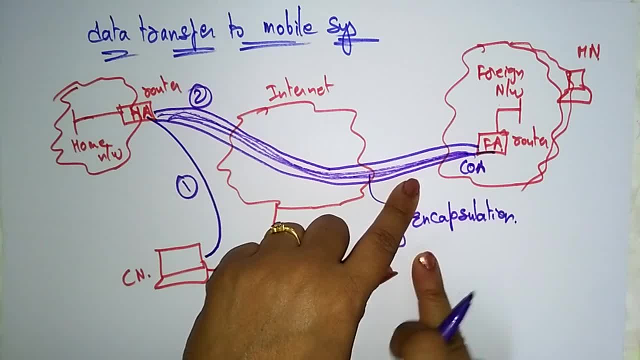 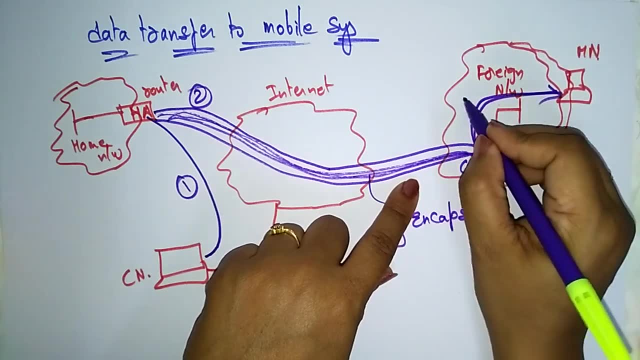 passing over the tunnel to COA by encapsulation, and next after that it is encapsulation, and next after that it is encapsulation, and next after that it is reaching to the mobile node 3. so the reaching to the mobile node 3, so the reaching to the mobile node 3, so the foreign agent forwards the packets to the 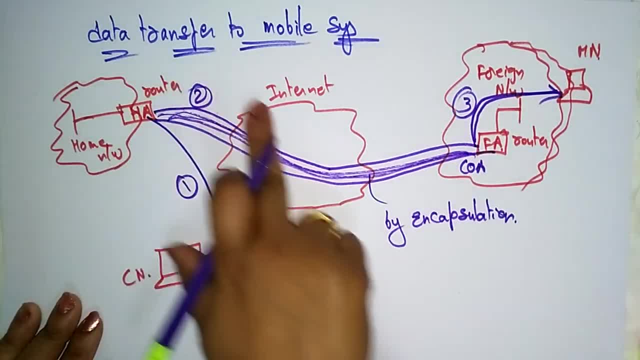 foreign agent forwards the packets to the foreign agent, forwards the packets to the mobile. no, so this is how the data is mobile. no, so this is how the data is mobile. no, so this is how the data is transferring to your mobile system, just transferring to your mobile system, just. 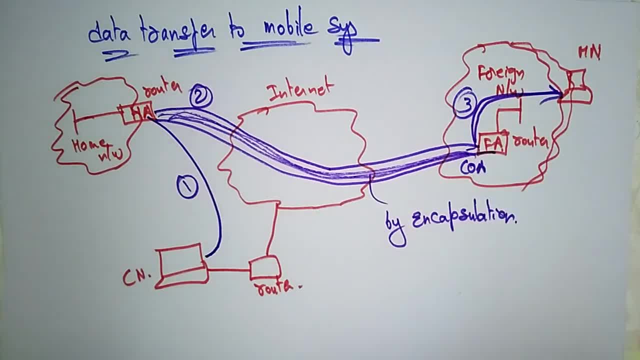 transferring to your mobile system, just it is transferring to your mobile system. it is transferring to your mobile system. it is transferring to your mobile system. so, in the same way, the data transfers. so, in the same way the data transfers. so, in the same way, the data transfers from the mobile systems. if you talk, 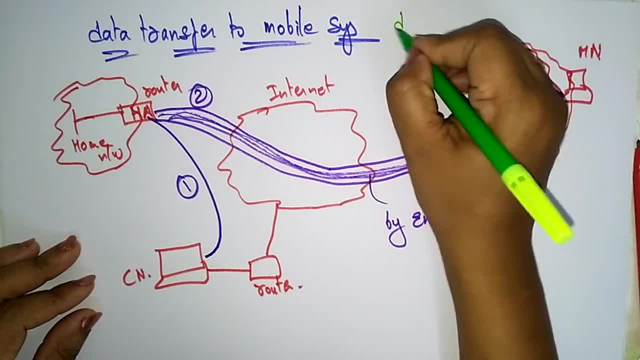 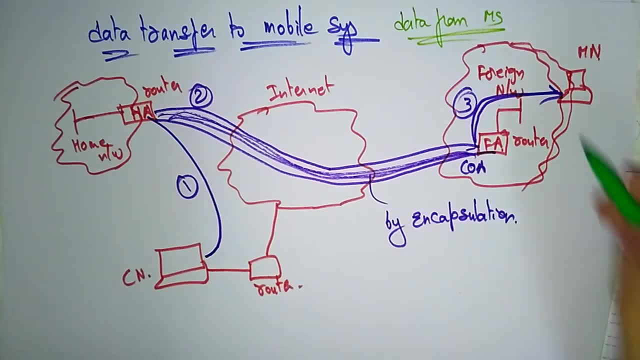 from the mobile systems. if you talk from the mobile systems, if you talk about from the mobile system, data from about, from the mobile system, data from about from the mobile system, data from mobile system. let me explain so first. mobile system. let me explain so first. mobile system. let me explain so first what it is doing: the mobile node sending